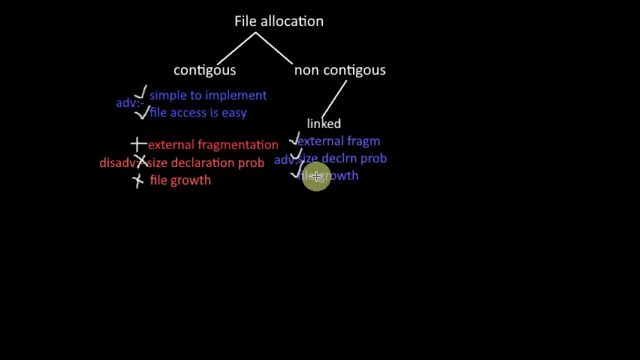 locations. But here the problem is the file access. The sequential file access is fine, but the direct file access is difficult. This method is not suitable for direct file access. Hence we go for the next method of non conditio allocation using file allocation table. 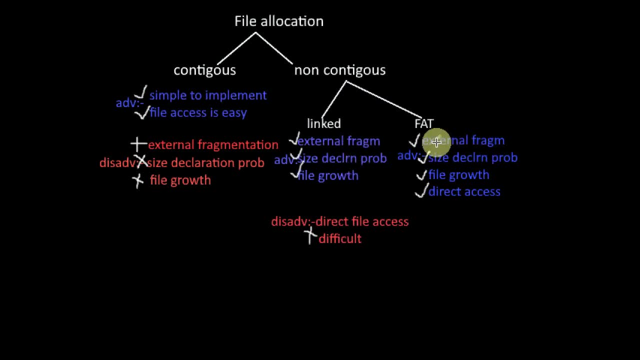 Here. all these advantages of linked allocation exist in this method. In addition, this method is suitable for both the sequential access as well as direct file access. But here we have a new problem: The size of the file allocation table. For every disk block we are having an entry in the file allocation table, Hence this table contain the details. 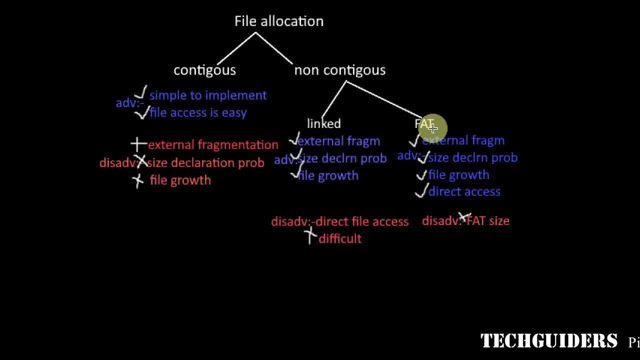 of not only the open files, also the files not in use, and it has the entries for the unused disk blocks too. We can get advantage from the file allocation table only if it's kept in the main memory while the disk is in use. If the size of the disk and the number 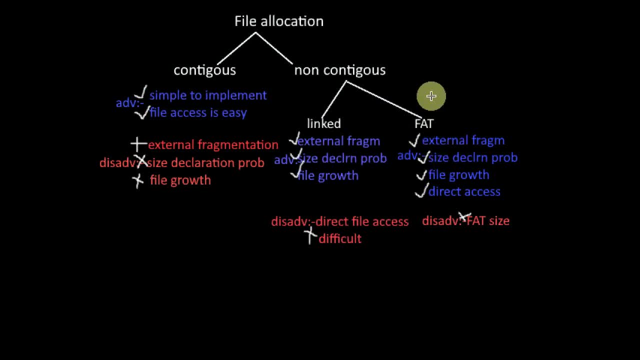 of disk blocks is very large. the file allocation table is too big and it's not fair to keep such a big table in main memory. So here we have the file allocation table. The file allocation table is too big and it's not fair to keep such a big table in main memory. 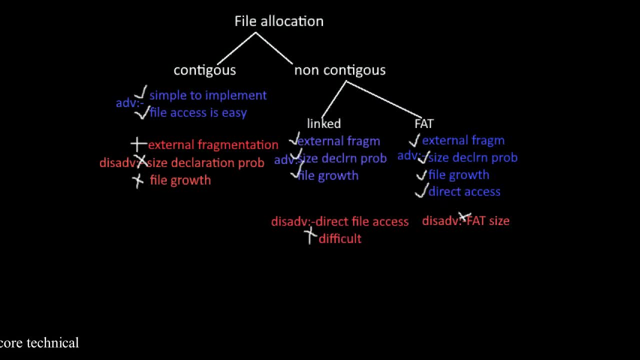 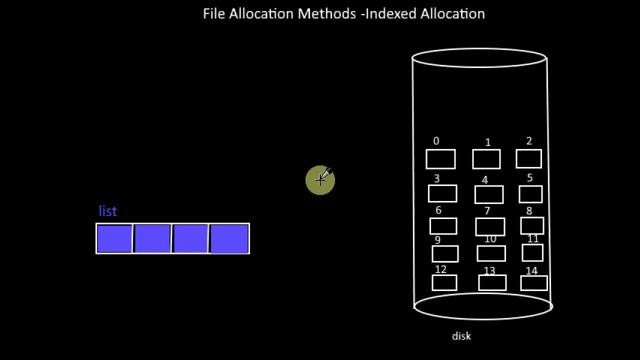 Thus, instead of using FAT we go for another non conditio allocation method called index allocation. Here the file is allocated with non conditio set of disk blocks, and for every file there will be a separate block called index block and the directory entry for that. 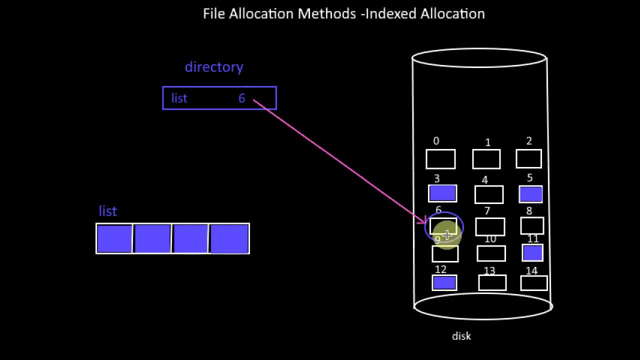 file points to the index block. So here we have the file allocation table. The file allocation table is too big and it's a bit life deutsing. The index block will then contain the location details of all the file blocks, or the pointers to all the file blocks, in order. The zeroth entry contains the value 3, which shows that 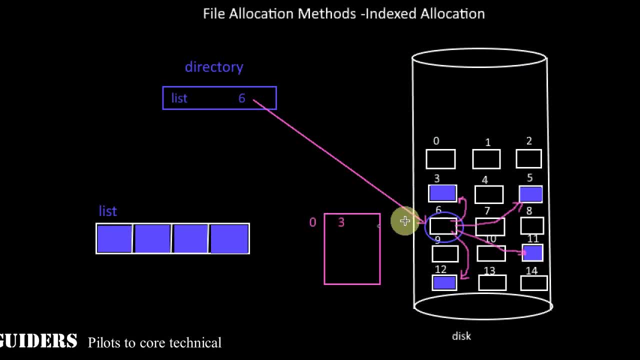 the first file block, or the zeroth file block, is at the location 3.. Then the next file block, the second file block is in the location 5 and the third file block as the disk block address 11, and the last file block has the disk block address 12..